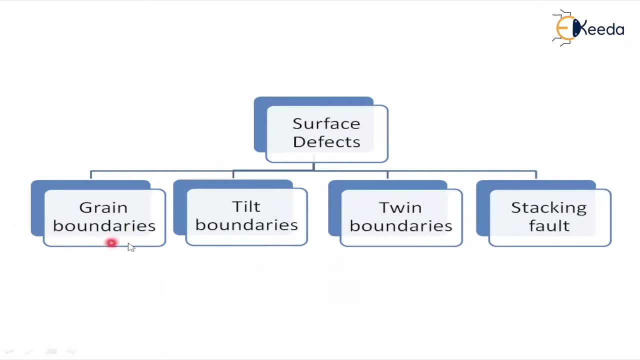 In this slide you are observing the four classifications: The classification under surface defects, grain boundary, tilt boundaries, twin boundaries and stacking faults. These tilt boundaries and twin boundaries come under grain boundaries. Before discussing the classification of surface defects, let us discuss what is surface defect, where it is formed, when it is formed. 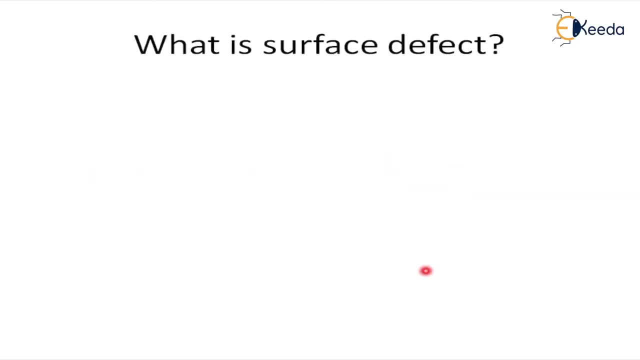 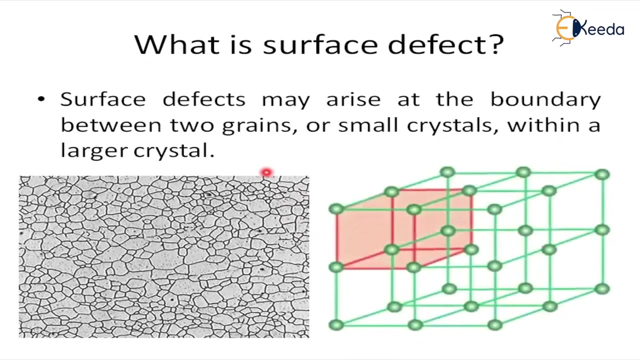 Here is the main point in this slide in surface defects. observe the surface defects may arise at the boundary between two grains, or small crystal within a larger crystal. so what it means, let me explain with the help of some figure here. so here you are observing two figures. we must know what is grain. 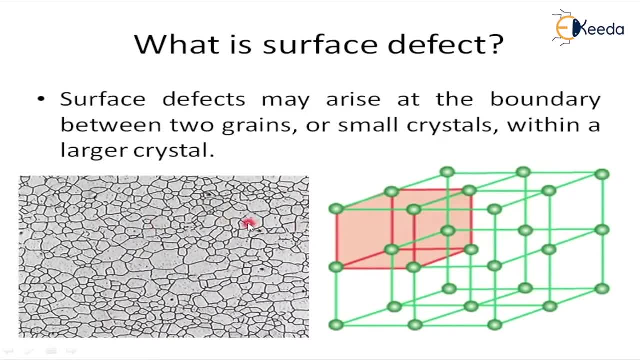 and what is crystal. these two images shows the grain boundaries and crystal lattice arrangement. the first image is the first image. the first image shows grains and grain boundaries. if a material surface observed under microscopic, that is, optical microscopic, the following grain boundary image will appear for better visibility we can observe: 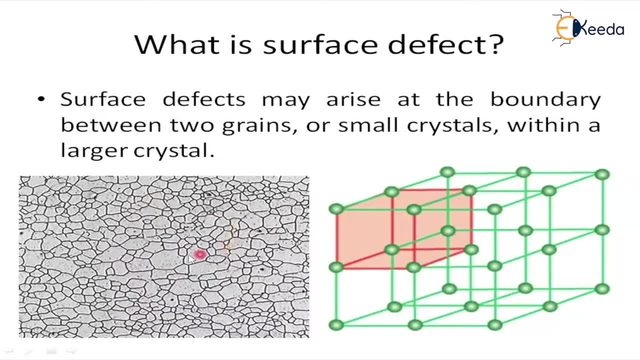 the surface of material under scanning electron microscope, with which we can inspect the grains and its boundaries with maximum magnification. here the second image shows. this is the unit crystal and this is a total crystal lattice structure. here this is called as a perfect crystal. perfect crystal means there is no dislocation in crystal lattice. in this slide you 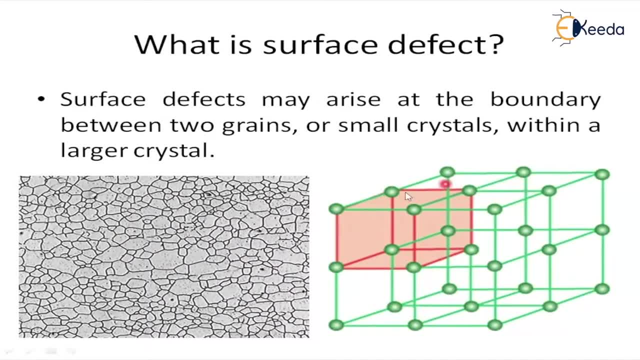 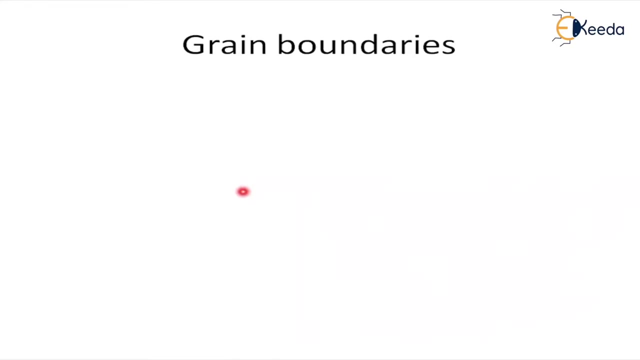 can observe the grain and grain boundary and crystal lattice. that means perfect crystal structure. let us discuss how the surface defect is formed and what do you mean by the surface defect and the classification in surface defects. the first type in surface defects is grain boundaries. let us discuss in detail. 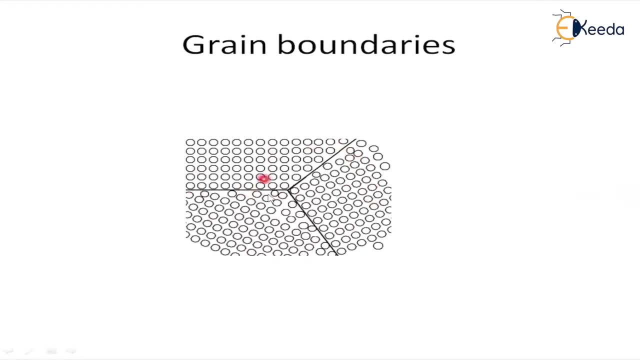 observe the image here. observe the image. this is the surface image. this is one grain. this is another grain. this is another grain on a crystalline solid here. observe this sentence here. crystalline solids are usually made of number of grains separated by grain boundaries, means the total crystalline solid made of number of grains like this. So many number. 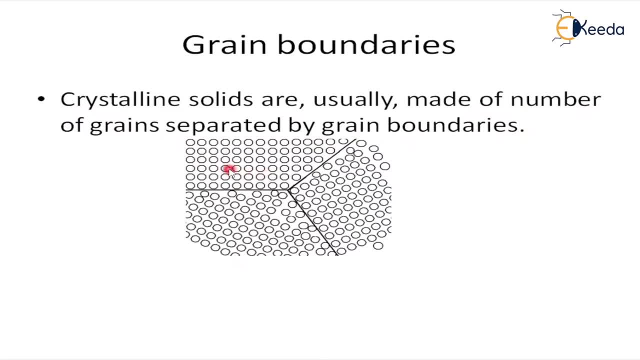 of grains, which is already observed in the previous slide. You can see here: this is one grain, two grain, third grain. So these type of grains may be existed and all these grains are separated with the help of grain boundary. This is grain boundary. This is very, very. 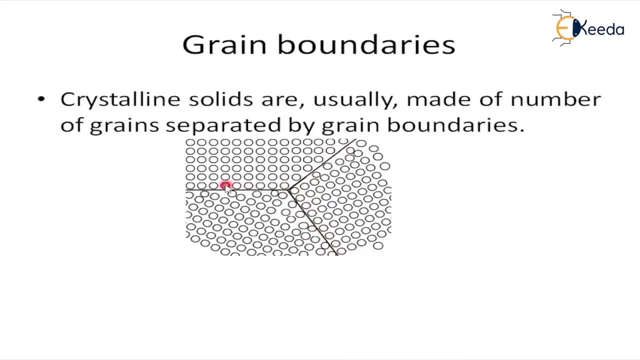 important. The boundary of the grain is important here. Now the two rows of atoms in two different grains may run in slightly different directions. If you observe here, this grain is having a different orientation and this atoms, all these atoms in this grain are having different. 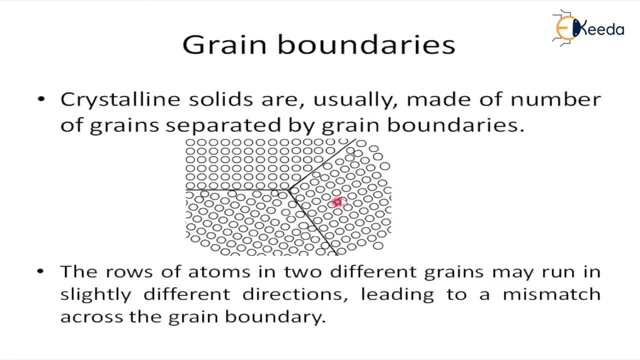 orientation and the atoms in this grain is having different orientation. So these two grains are having different variations and they have different orientation of the grain. So that means all these grains are not having the same orientation, Each and every grain. so this grain is having, suppose say, horizontal and this grain is having some inclination and 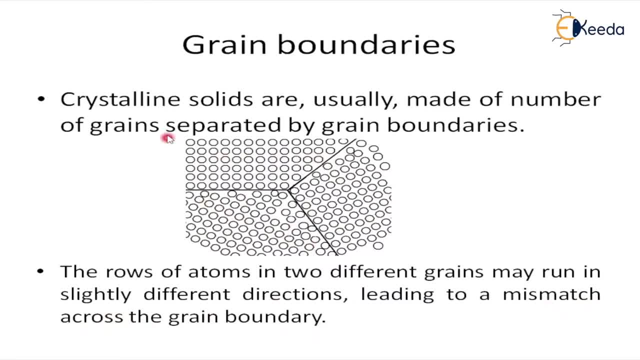 this is having some other inclination. If this is the arrangement, then it leads to a mismatch across the grain boundary. Now we are discussing why this happened. what do you mean by grain boundary defect? The grain boundary is a different boundary, If you see. 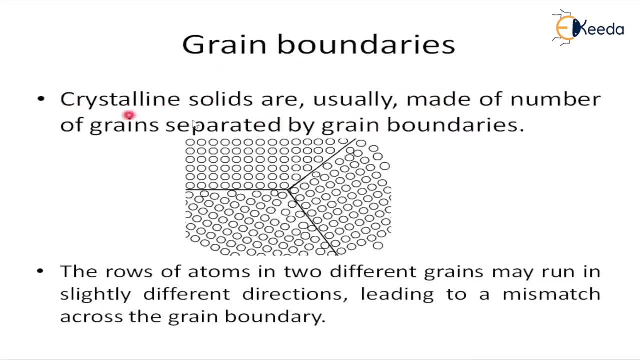 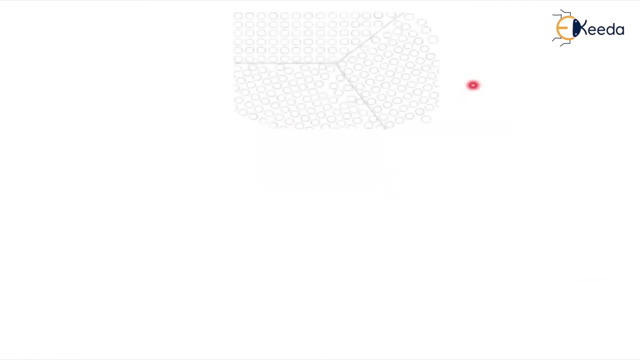 on the surface in crystalline solid. now, if the grains are like this, if the atoms are arranged like this, then we can call that as a mismatch and which leads to a grain defect, which is represented as a grain boundary defect. now let us see some more points here. when this misalignment is slide on the order of: 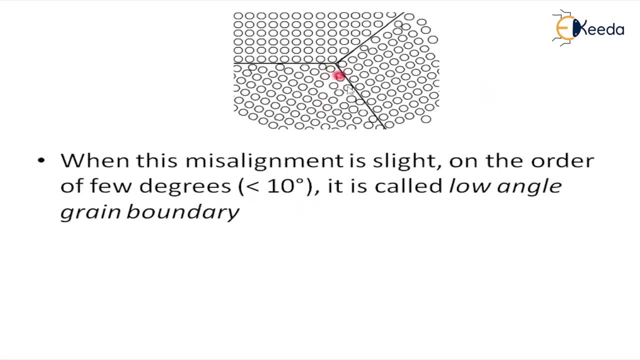 few degrees, suppose, say less than 10 degrees. this angle between this and this, if it is an order of that, is few degrees, less than 10 degrees. we can say it is called as low angle grain boundary. these boundaries can be described in terms of aligned dislocation arrays. suppose if 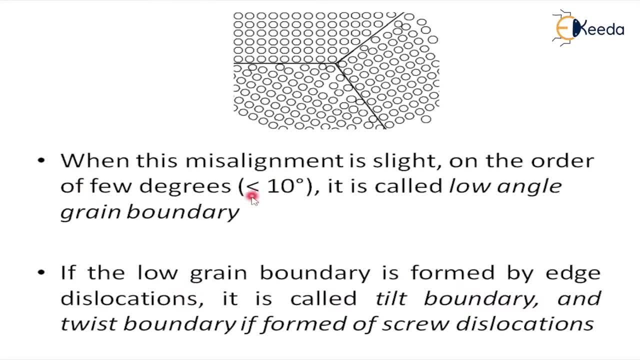 the low grain boundary is formed. that means if it is less than 10 degree, the angle is less than 10 degree, then it is called as a low grain boundary. if it is formed by edge dislocation, it is called tilt boundary, and fist boundary means if 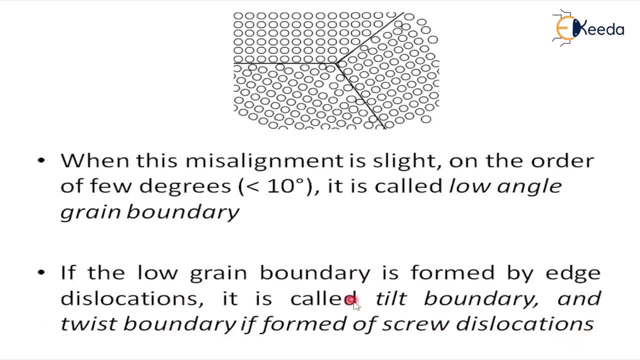 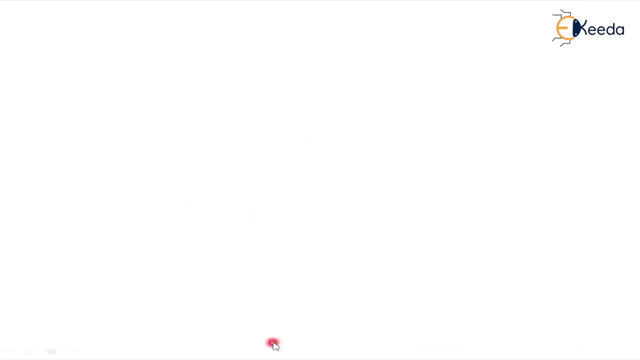 it is formed with screw dislocation, so that means in edge location. if the grain boundary is formed in edge location, that is called as a tilt boundary. if it is formed in screw dislocation, that is called as a twist boundary. we will learn some more features in tilt and twist boundary here. this is the main point: both tilt and twist boundaries. 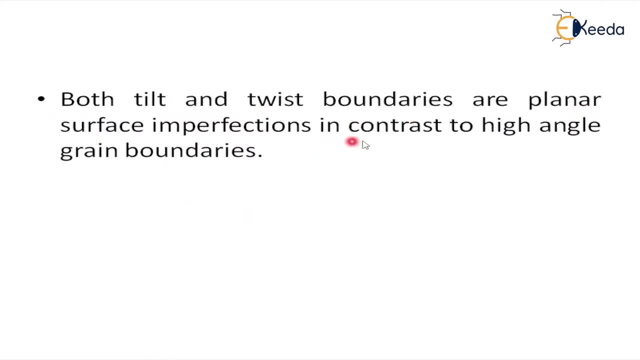 are planar surface imperfections, in contrast to high angle grain boundaries. what do you mean by high angle grain boundaries here if the angle is less than 10 degree? we already said that it is low angle grain boundary. what do you mean by high angle grain boundary if? 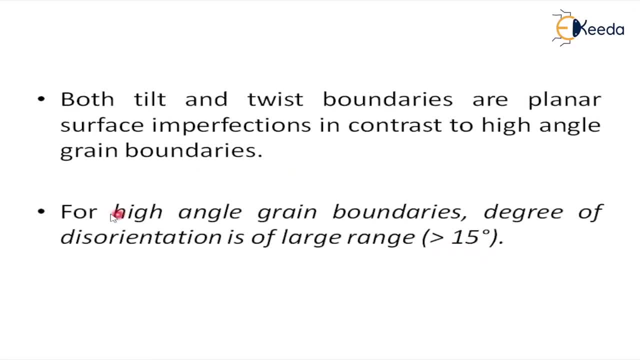 the angle is greater than 15 degree. so that means high angle grain boundary means if the orientation is greater than 15 degree, then we can say that it is high angle grain boundary. in general, grain boundaries are chemically more active because of grain boundary energy. 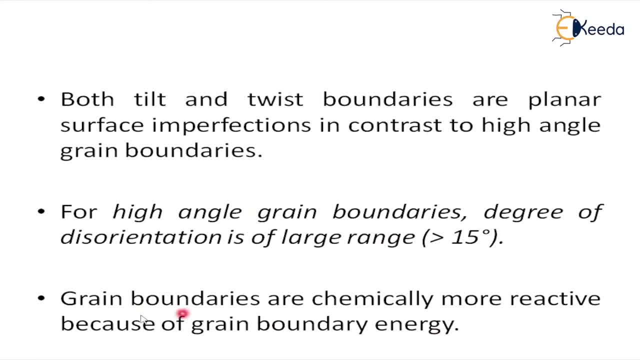 If the energy is more for a crystalline solid means the grain boundaries are having chemically active. That's why the surface is more active. If the surface is not active, we cannot form a chemical reaction with other material. So that's why this is a very, very important analysis and important ideology and important information. 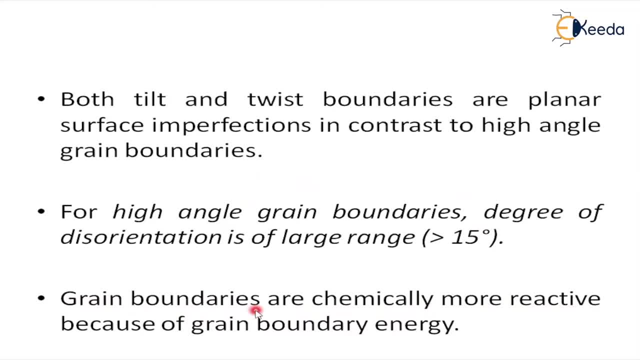 with which we can clearly say that with which material it is going to have chemical reaction. So that's why we are studying grain boundaries. If grain boundaries are not reactive, we cannot say that this material is going to act with some other surface or some other material. 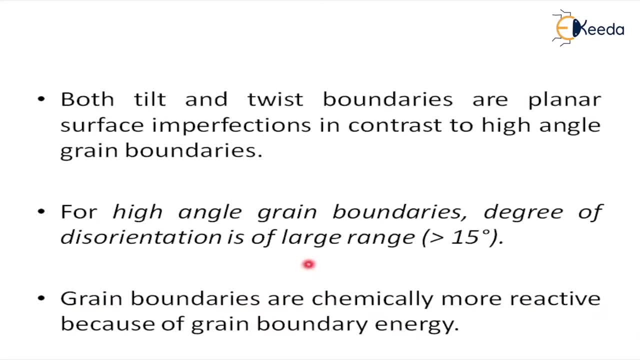 Now let us discuss twin boundary. Before going to discuss twin boundaries, one more information. with tilted twin boundary, In spite of disordered orientation of atoms at grain boundaries, polycrystalline solids are still very strong as cohesive forces present within across the boundary. 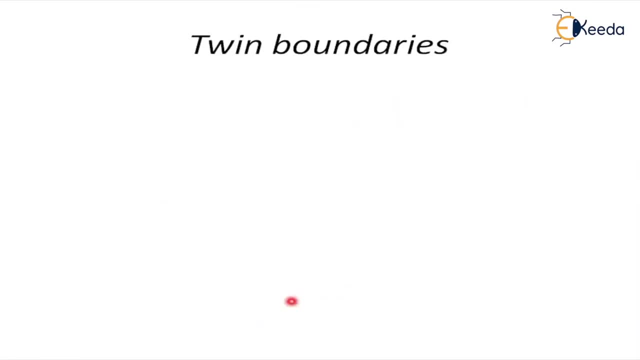 Now let us discuss twin boundary. What is twin boundary? Please observe the image here, observe the image carefully here. this is one surface, this is same surface, same plane, but a region is deformed. here, some of the region is deformed. this is first boundary. this is second boundary. 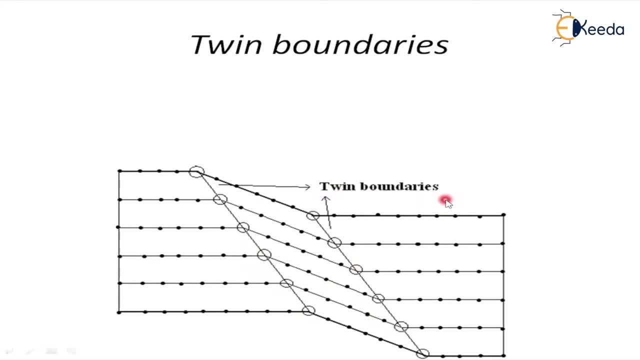 Now, what do you mean by twin boundary here? It is a special type of boundary. It is a special type of boundary. It is a special type of grain boundary across which there is a specific mirror lattice symmetry. You can observe this is similar to this. 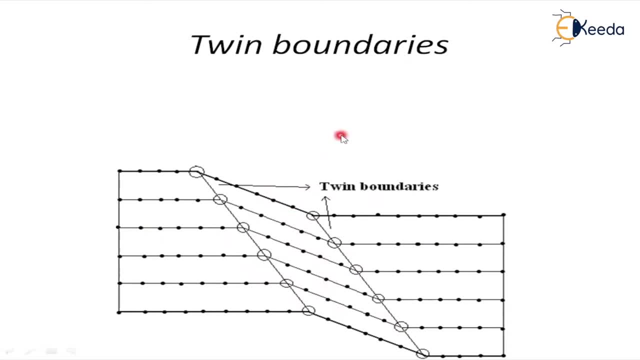 So this acts as a mirror. It is observed in the image that twin boundaries occurs in pace such that the orientation change introduced by one boundary is restored by the other. So that means if any deformation is observed Here, it is restored by the other. 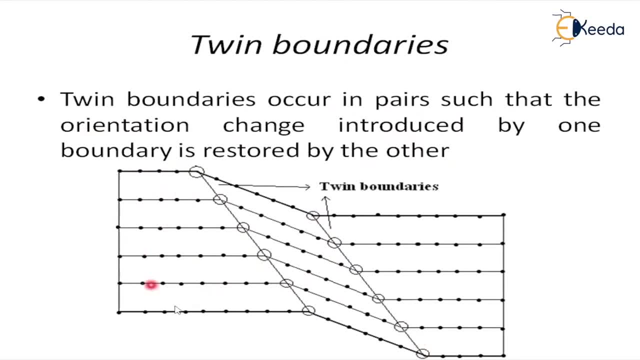 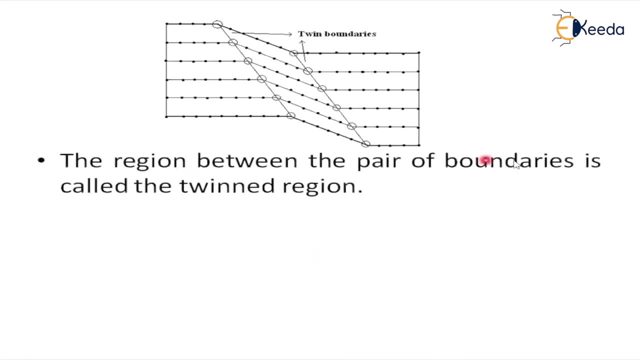 Again, the same type of surface and same type of arrangement is again restored after some region, This is called as a twin boundary. The main salient features of twin boundary is the region between the pair of boundaries is called the twin region. So that means this is the first one. 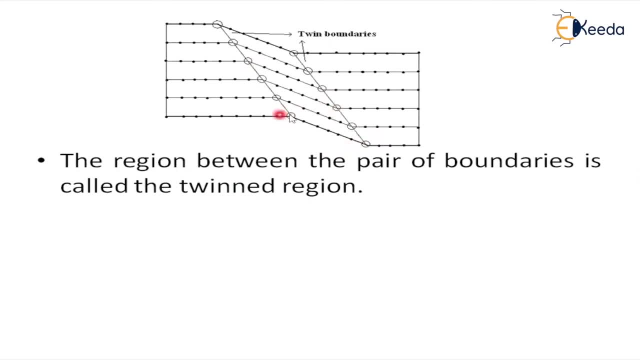 This is second. one is the first region, is the second Is the region Between the pair of boundaries. So this is the first one and second. These two are called as a pair of boundaries, is called as a twin region. Just observe the twin region here. 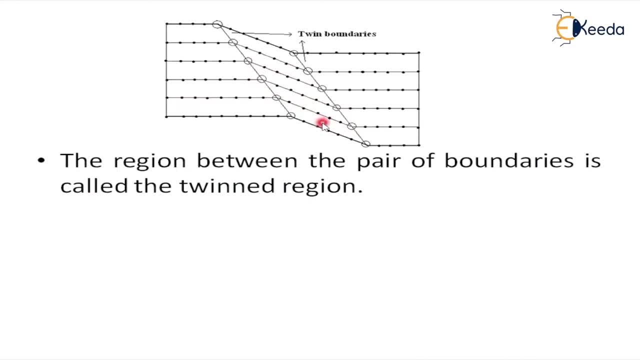 This is the twin region. If twins which forms during the process of recrystallization, then it is called as annealing twins, Whereas deformation twins form during plastic deformation Means depends on the process. twin region will become either annealed or deformation twin. 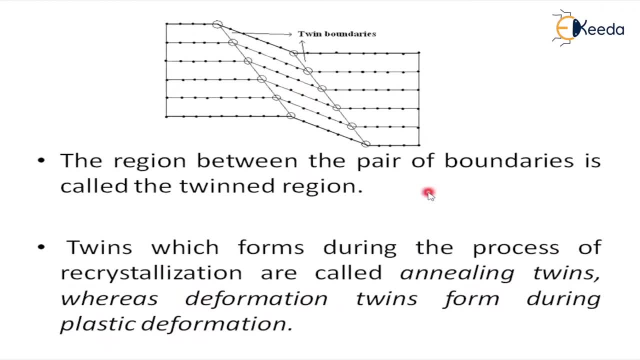 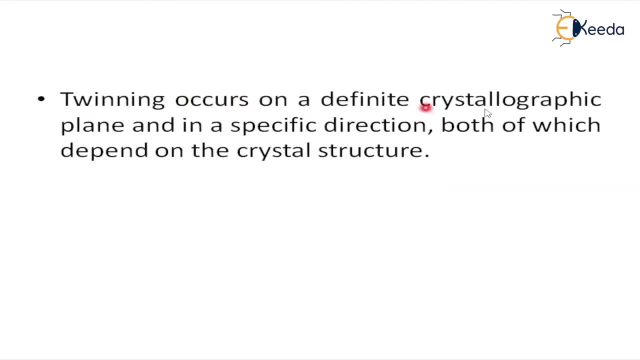 So that means permanent deformation twin. Here we will observe some salient features. Twinning occurs on a definite crystallographic plane and in a specific direction. Here the important point in twinning is It observed In a specific direction, Both of which depends on the crystal structure. 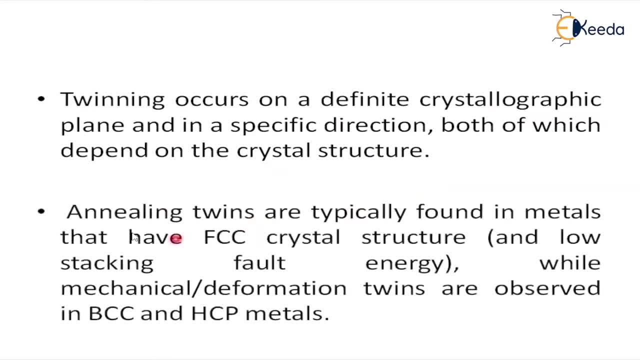 Here two points. I already said that annealing and permanent annealing twins are typically found in metals that have FCC crystal. Most of the annealing twins are formed in FCC crystal structure and because they are having low stacking fault, And this is the main reason why the annealing twins formed in FCC crystal structure. 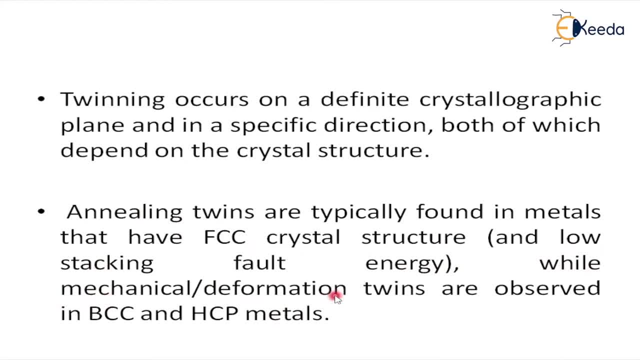 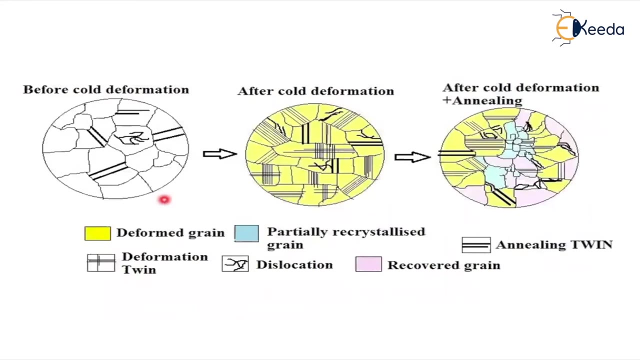 While mechanical deformation, Deformation, That means permanent deformation or plastic deformation. twins are observed in both VCC and HCP crystals: Body centered cubic and hexagonal centered plastic metals. So face centered cubic metals is best example for annealing twins Now. 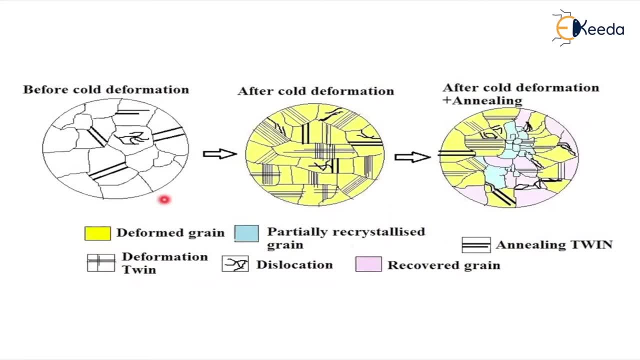 This image shows the schematic illustration of progressive twin density Obtained after cold working. That is, cold rolling here, Cold Before cold deformation. This is the microstructure After cold deformation. This is the microstructure If we add annealing. 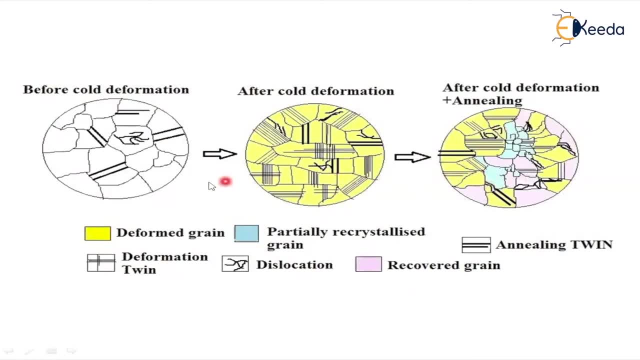 This is the microstructure. It also reveals sub micron grain associated with the deformation twins after annealing. Some regions are permanent. Some regions are permanently deformed, Represented as a deformation twin, Deformation twins. So this is deformation twin. 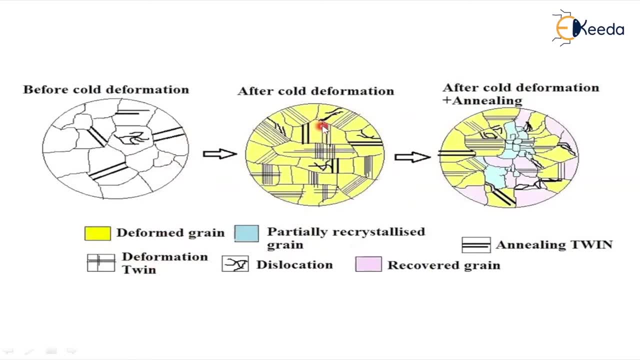 Is a deformed grain, A low color And twins here. This color is a recovered grains Is the annealed region. Annealed region means it may recover in future. These annealing twins are not permanent deformation. This may recover after some stresses. 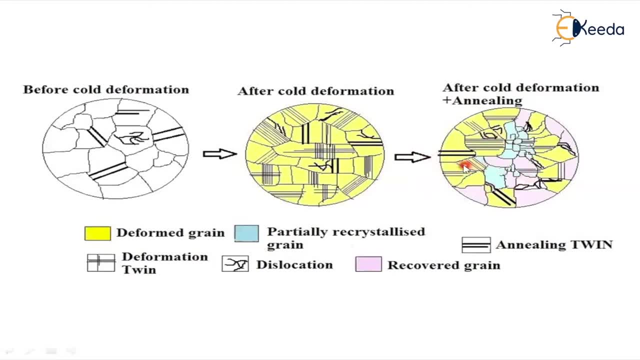 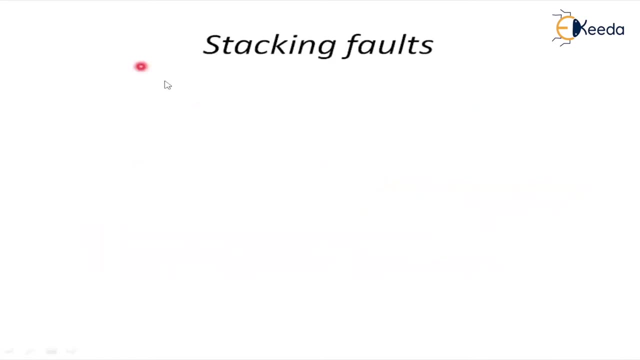 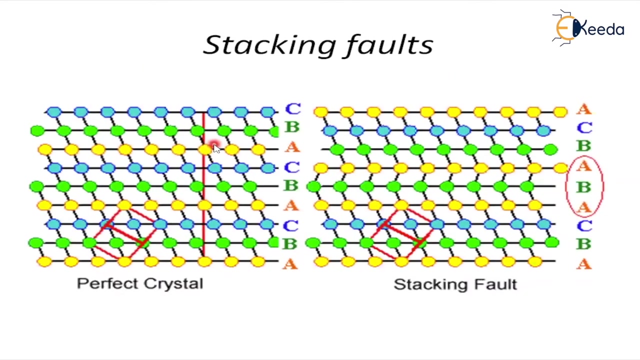 Annealing twins are usually broader and with a strider size, like this Strider size than mechanical twins, And twins do not extend beyond a grain boundary. Let us observe the last classification: Stacking faults. Observe here They are faults in stacking sequence of atomic planes. 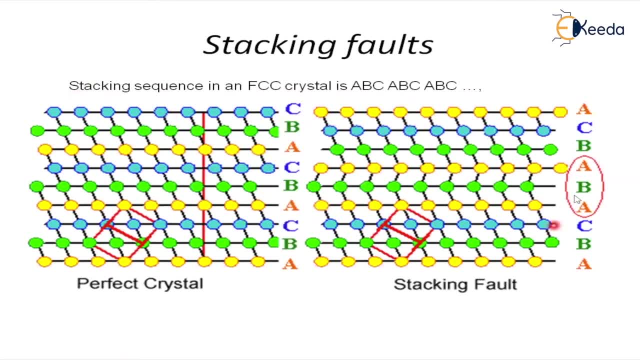 Stacking sequence in an FCC crystal. Here I have taken an example of FCC. The stacking sequence in an FCC crystal is ABC, ABC and ABC. Like this, This is a perfect crystal. Left side of the figure You are observing as a perfect crystal. 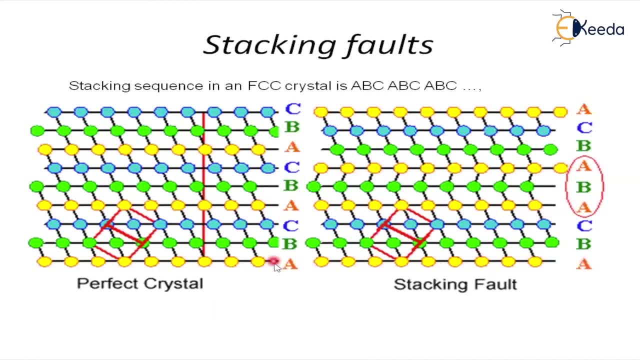 Right side is the fault. If you observe ABC here, ABC here, This is a perfect crystal. But here, After ABC, A, B, A, Here this is the fault. Again B, C, A, So like this: 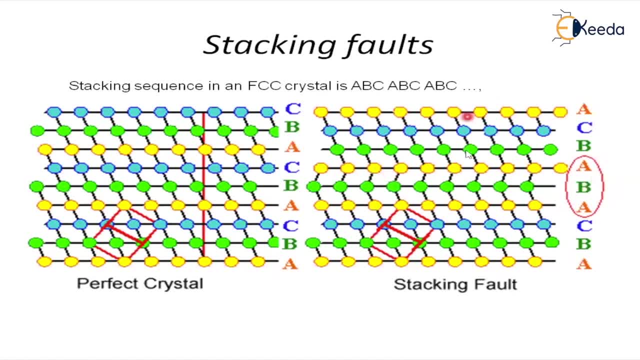 The total stack, All the layers are disturbed And this A is represented as a stacking fault. When the disturbance in stacking sequence, Deformation of stacking faults takes place. Now, The lower The stacking fault. energy, Wider the stacking faults. 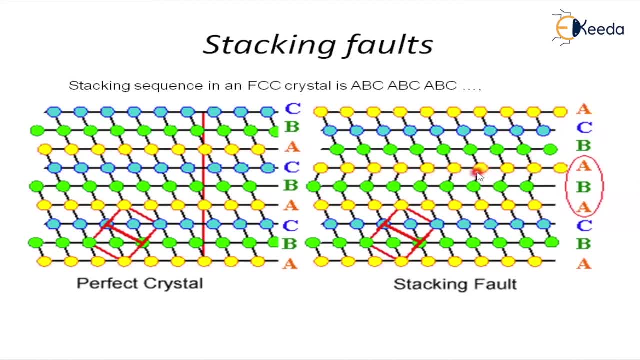 Suppose, if the energy is very lower, Then stacking fault is also wider. Metal strains hardens rapidly And fiend is like this. You can observe It is fiend Because of this disturbance. It is fiend That is a narrower stacking faults.